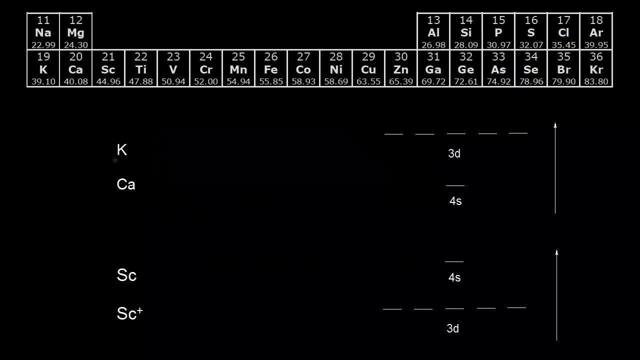 We've already looked at the electron configurations for potassium and for calcium, but let's do it again really quickly, because it's going to affect how we think about the d orbitals. We find potassium, which is in the fourth period on the periodic table, and if we do, 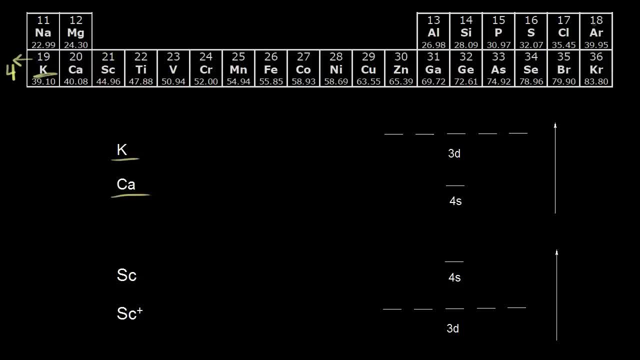 noble gas notation. to save some time we work backwards and the first noble gas we hit is argon. We write argon in brackets. We know argon has 18 electrons and potassium has 19 electrons, so potassium has one more electron than argon. We put that extra electron into a 4s orbital, because for potassium the 4s orbital is lower energy than the three d orbitals here. so we have increasing energy and that electron goes into a 4s orbital. so the complete electron configuration. 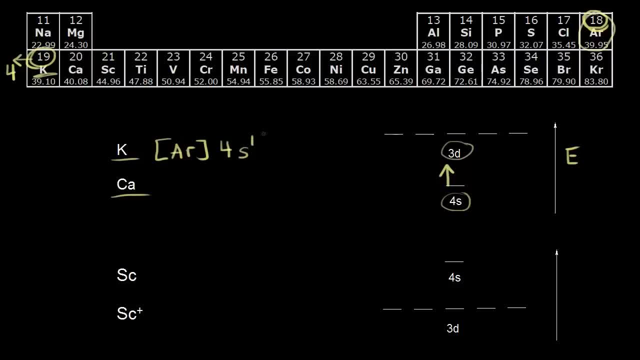 using noble gas. notation for potassium is argon in brackets 4s1. For potassium, for calcium I should say we have one more electron than potassium, and so that electron's going to go into the 4s orbital as well. 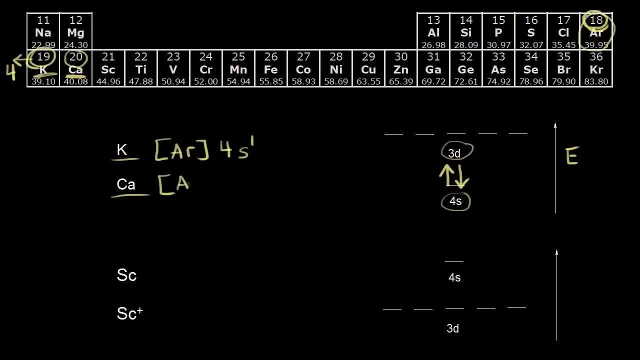 We pair our spins and we write the electron configuration for calcium as argon in brackets 4s2.. For the calcium 2 plus ions, if you think about forming an ion, here we're talking about the electron configuration for a neutral atom, meaning equal numbers. 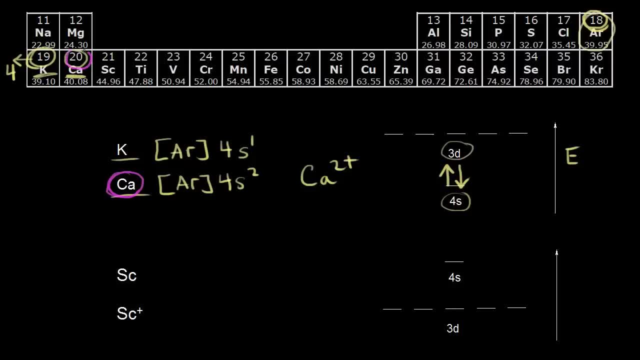 of protons and electrons, With an atomic number of 20, 20 protons and 20 electrons. If we lose two electrons, we have a net positive 2 charge, so we form the calcium 2 ion, The two electrons that we would lose. 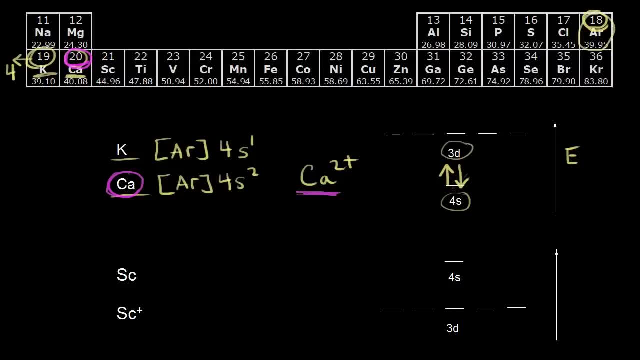 to form the calcium 2 plus ion. are these these two electrons right here in the 4s orbital? The electron configuration for calcium 2 plus would be the same as the electron configuration for the noble gas argon- here For potassium, once we accounted for argon. 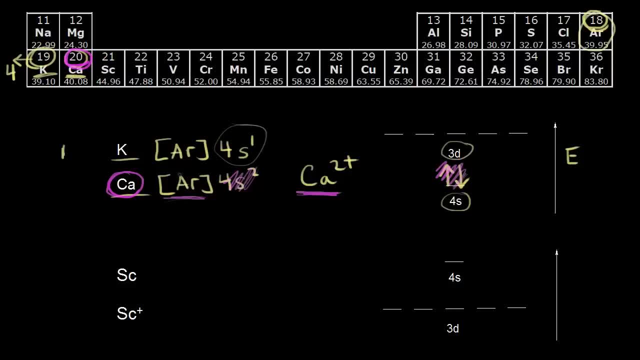 we had one electron to think about For calcium. once we accounted for argon, we had two electrons to think about. If we go to the next element on the periodic table, that's scandium, That's one more electron than calcium. 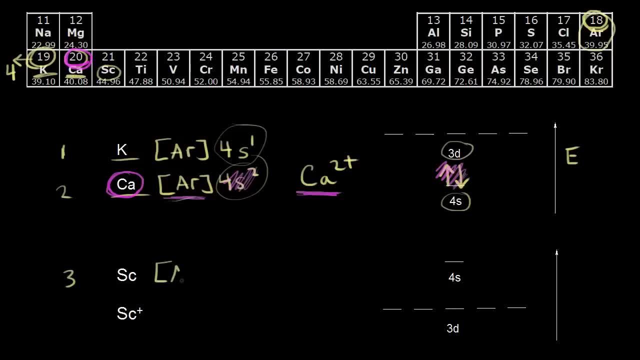 so we'd have three electrons to worry about once we put argon in here like that. This is where things get weird. Now we have to think about the d orbitals, and once again things are very complicated once you hit scandium, because the answer 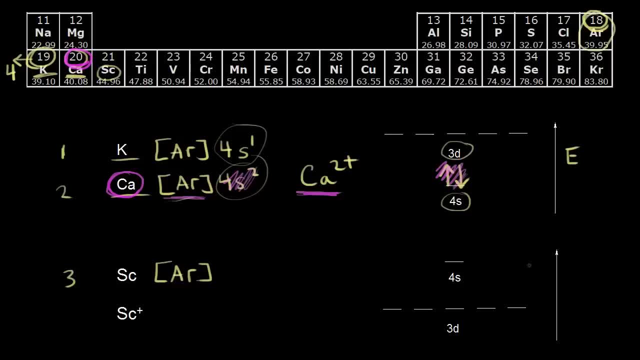 is energies change When you hit scandium, even though these are very small energy differences- now the energy of the 4s orbital is actually higher than the energy of the 3d orbitals- We're talking about, once again, increasing energy. 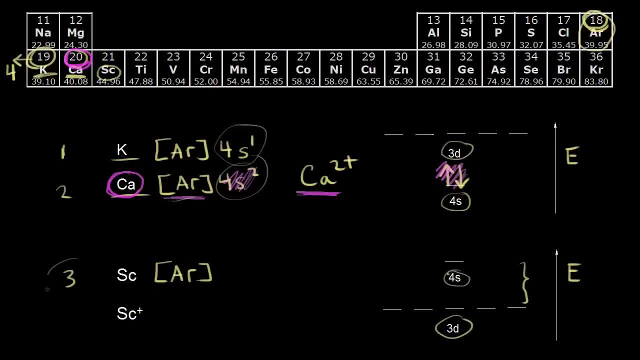 That's pretty weird. If you think about these three electrons, where are we going to put them? Your first guess if you understand these energy differences might be: I'm going to follow Hund's rule. I'm going to put those electrons in the lowest. 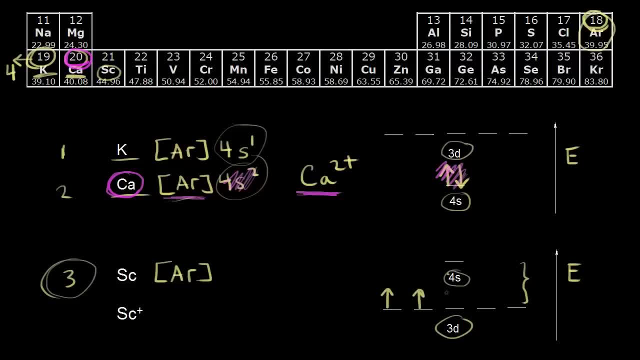 energy level possible here. I'm going to not pair my spins, so I'm going to write my electron configuration like that for scandium. You might think it would be argon 3d3.. That's not what we observe for the electron. 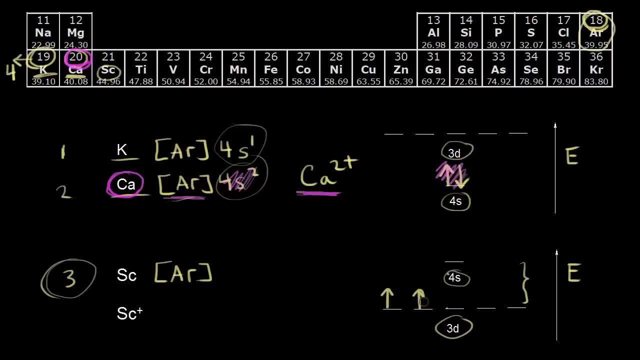 configuration for scandium. Actually, two of these electrons actually move up to the higher energy orbital. Two of those electrons move up to the 4s orbital here, like that, The electron configuration turns out to be 4s2, 3d1.. 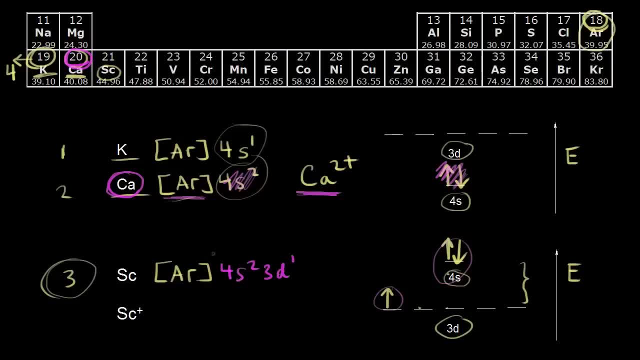 It's actually 4s2, 3d1.. Or, if you prefer, 3d1, 4s2.. Once again, with argon in front of it. Either one of these is acceptable. This is weird. Why do those electrons? why do those two? 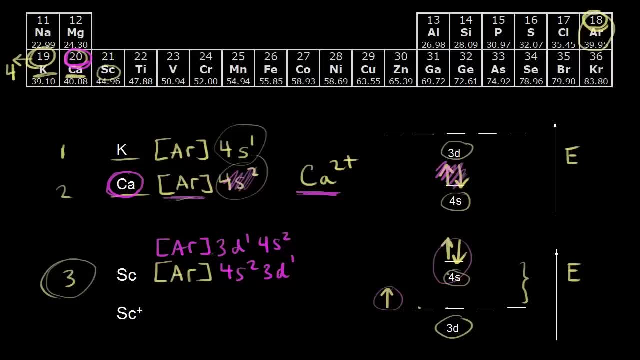 electrons go to an orbital of higher energy. There's no simple explanation for this. Even though it might be higher in energy for those two electrons, it must not be higher energy overall for the entire scandium atom. There are many other factors to consider. 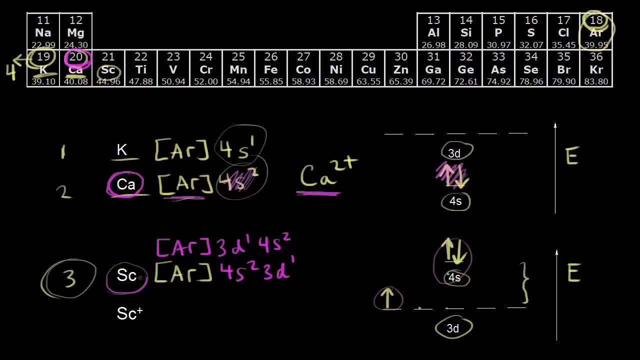 Things like increasing nuclear charge. Scandium has an extra proton compared to calcium. Then there are once again many more factors and far too much to get into in this video. Unfortunately, there is no easy explanation for this. This is the observed electron configuration. 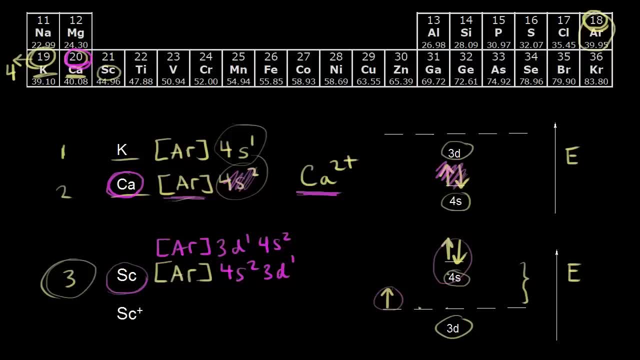 for scandium. How do we know this is true? How do we know that the 4s orbital is actually higher energy than the 3d orbitals? We know this from ionization experiments. For example, if you form the scandium plus one ion. 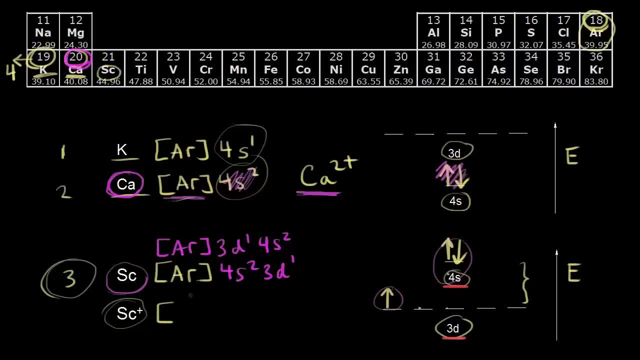 the electron configuration for the scandium plus one ion. so we're losing an electron from a neutral scandium atom. this turns out to be argon 4s1, 3d1.. Once again, you could write argon 3d1, 4s1.. 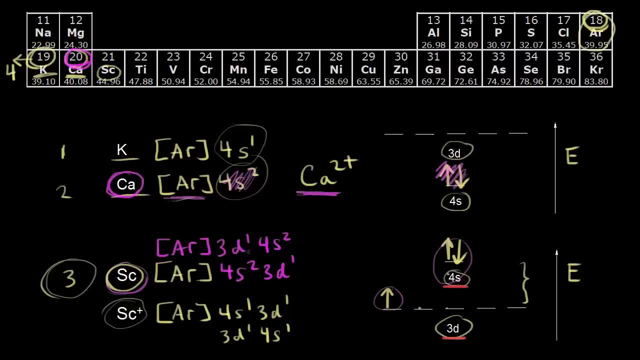 Where did we lose that electron to form our ion? We lost that electron from the 4s orbital. We had 4s2 here and here we have 4s1.. We lost this orbital, We lost this electron. That only makes sense if the 4s orbital is the highest. 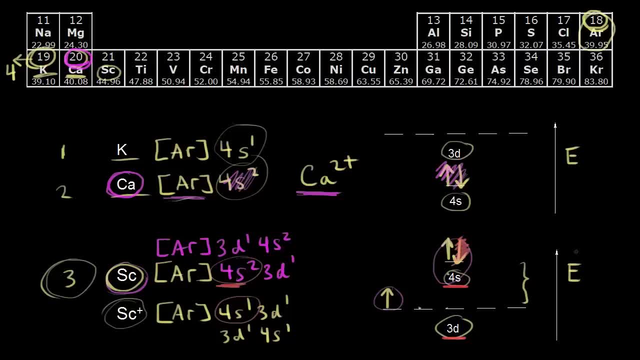 in energy, because when you lose an electron for ionization, you lose the electron that's highest in energy. That's the one that's easiest to remove to form the ion. The 4s orbital is actually higher in energy than the 3d orbitals. 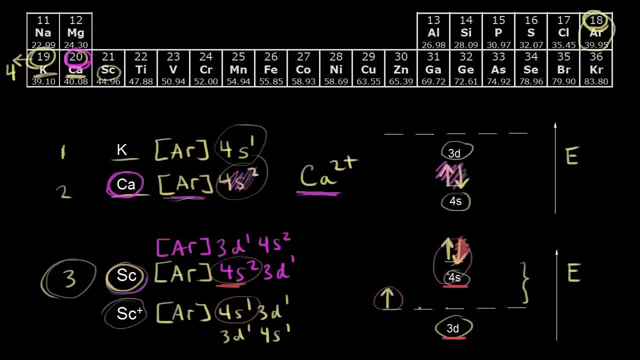 You don't see this a lot in textbooks. I think the main reason for that is because of the fact that if you're trying to think about just writing electron configurations, your goal is to write. Let's say, you're taking a test and your goal is to write. 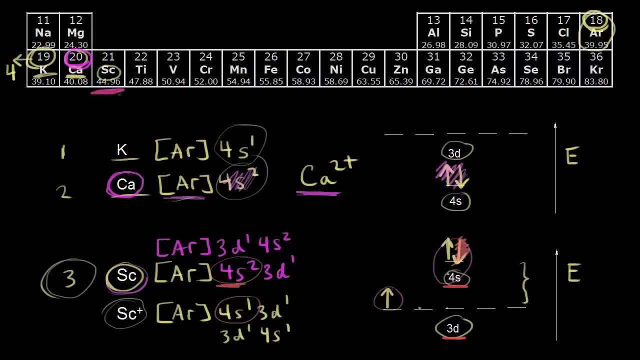 the electron configuration for scandium. The easiest way to do that- Let me go ahead and use red here. The easiest way to do that. if you want to write the electron configuration for scandium, you look at the periodic table and if you're doing noble, gas notation. 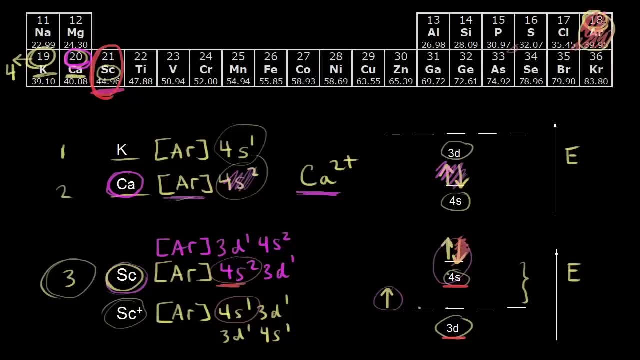 the noble gas that precedes. it is of course argon right here That takes care of the argon portion. Then, looking at the periodic table, you would say this could be 4s1,, 4s2,, 3d1,. 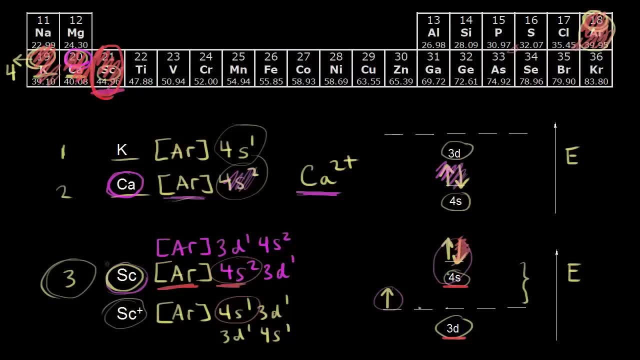 and so on. That gives you the correct electron configuration: argon 4s2, 3d1.. It's implying that the d orbitals, the 3d orbitals, fill after the 4s orbital and is therefore a higher energy. 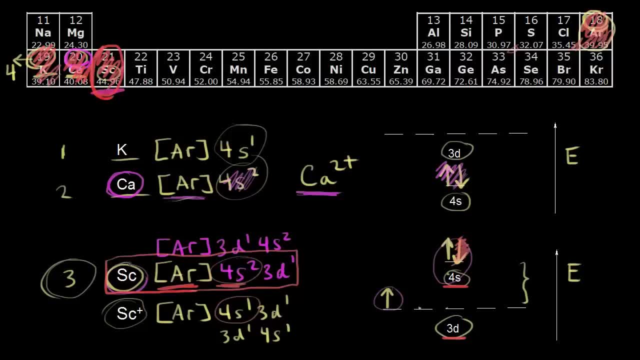 That's not true. actually, It does help you to just assume that's the case if you're writing an electron configuration, but that's not what's happening in reality. We need to think about the other elements here. We just did scandium. 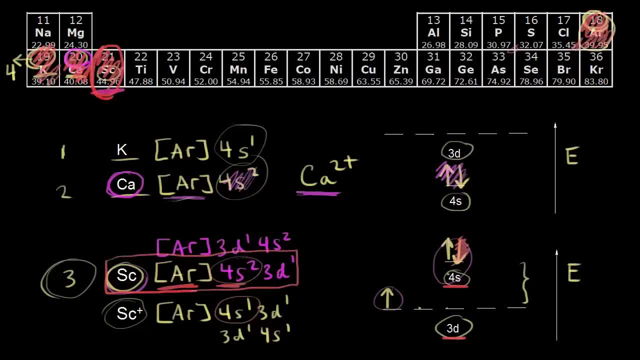 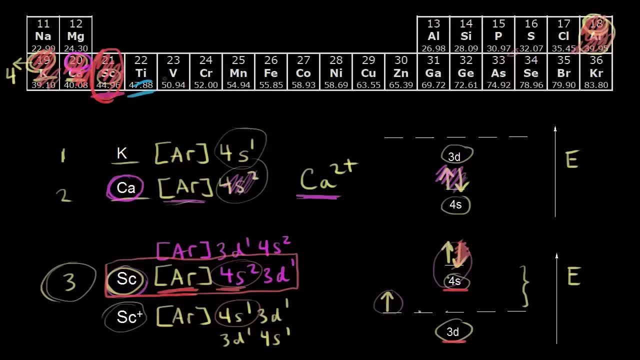 Next, let's move on to titanium. Thinking about titanium, the next element in the periodic table, if your question on the test was write the electron configuration for titanium, the easiest way to do it is just once again to think about argon. 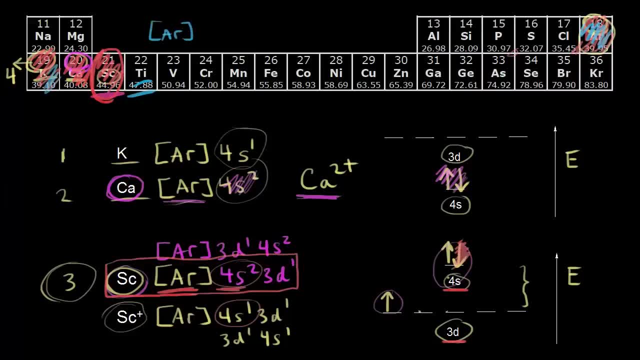 Put argon in brackets and then think to yourself: this would be 4s1,, this would be 4s2,, this would be 3d1, and this would be 3d2.. 4s2, and then 3d2.. 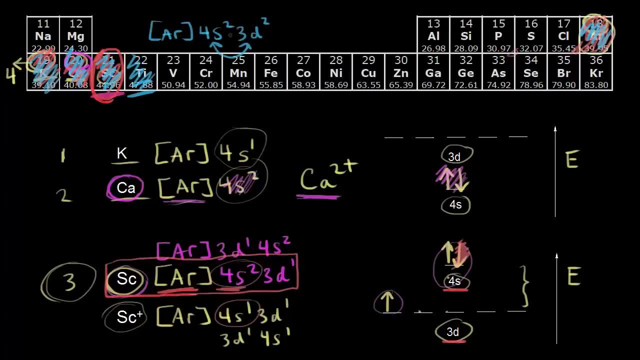 Once again, you could switch 3d2 and 4s2.. Once again, this is implying the d orbitals fill after the 4s orbital, which isn't true, but it does get you the right answer. It's useful to think about it both ways. 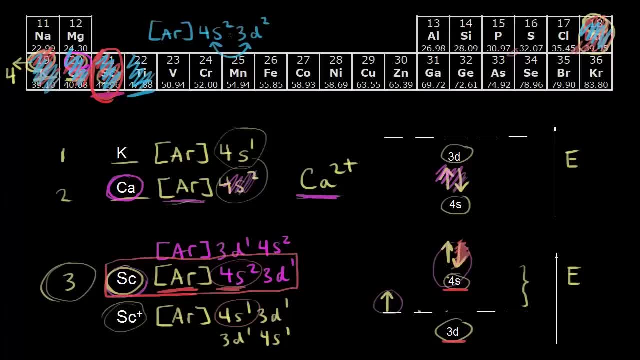 It's useful to think about the energy levels properly, but at the same time, if your goal is to get the answer the fastest way possible, looking at the periodic table and running through the electron configuration might be the best way to do it on a test. 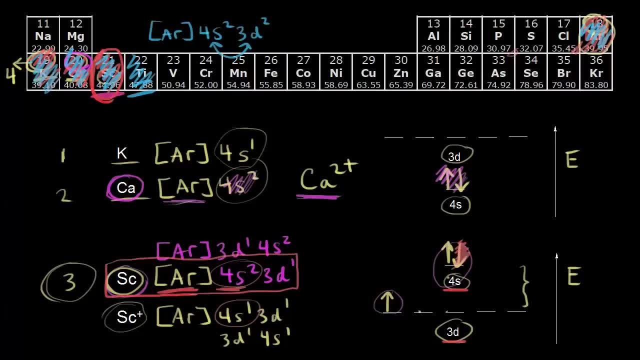 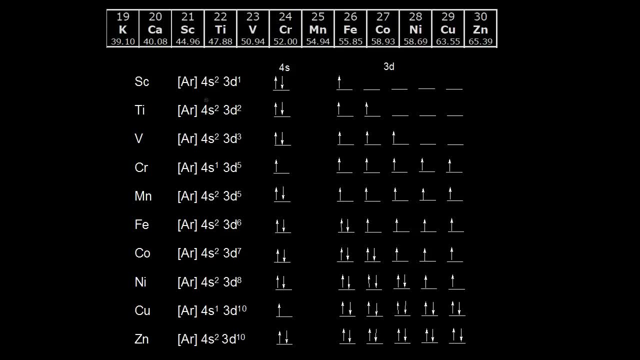 Let's look at some of these other elements here. We've just talked about scandium and titanium. Let's go down here and let's look at this little setup here. We just did scandium and titanium. Scandium was argon 4s2, 3d1.. 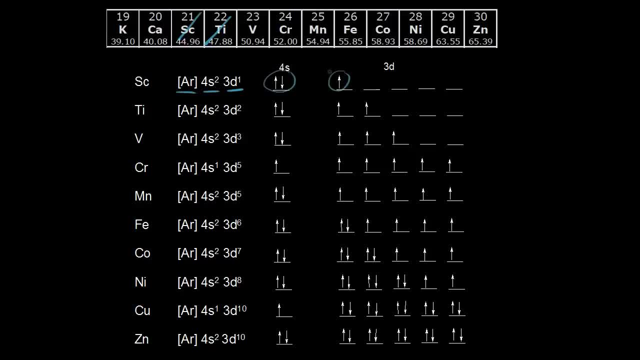 We talked about two electrons in the 4s orbital, one electron in the 3d orbital, and then we just did titanium 4s2,, 3d2, or, once again, you could switch any of these When you're doing orbital notation. 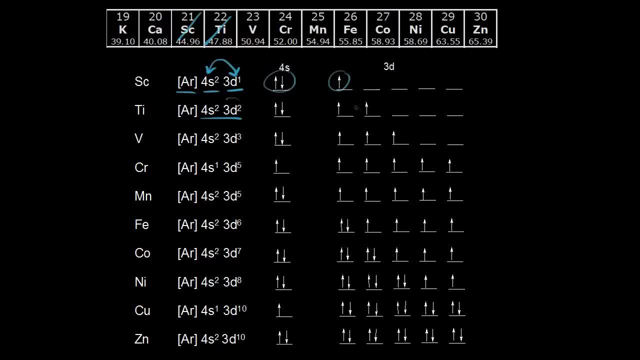 adding that second electron to a d orbital. here's the electron that we added, so we didn't pair up our spins. We're following Hund's rule here. Next element is vanadium, so we do the same thing. One more electron. 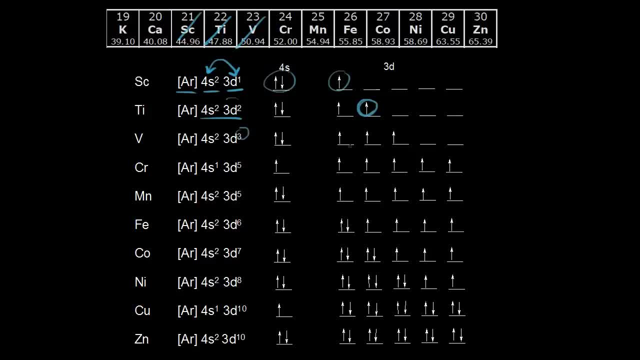 We add that electron to a d orbital, but we don't add it to one of the ones that we've already started to fill here. We add that electron to another d orbital, Once again, following Hund's rule: Things get weird when you get to chromium. 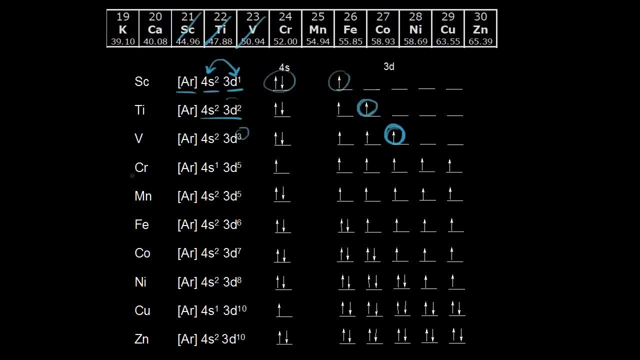 Let me use a different color here for chromium. Just thinking about what might happen for chromium. Chromium- one more electron to think about than vanadium. You might think let's just add that one electron to a 3d orbital like that. 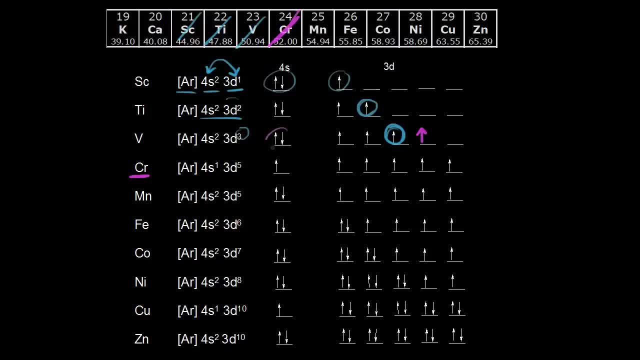 and then be done with it. If you think about it, you might guess 4s2, 3d4.. Let's go ahead and write that 4s2, 3d4, so question mark. That's not actually what we get. 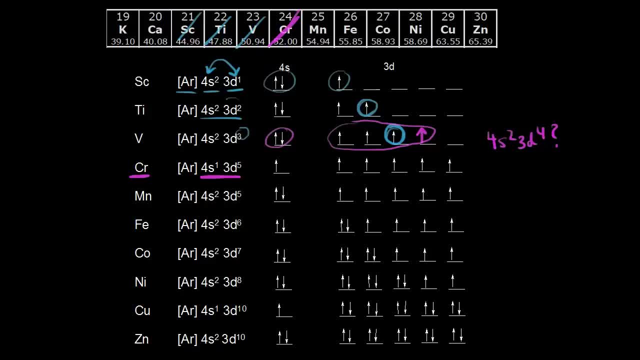 We get 4s1, 3d5.. That electron, this electron. here Let me go ahead and use red. You can think about this electron. We expected it to be there. We expected it to be 4s2, 3d4. 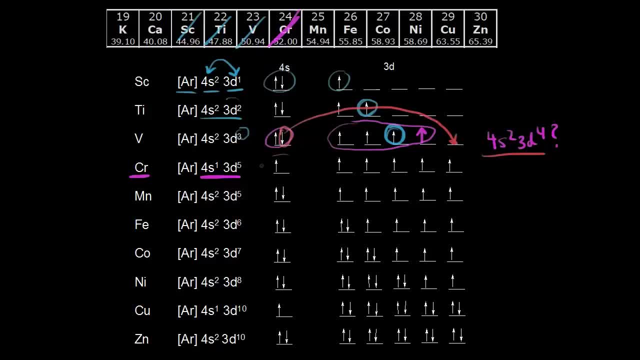 It's like that electron has moved over here to this empty orbital. to give you this orbital notation. That's just an easy way of thinking about it. In reality, that's not what's happening if you're building up the atom here, because of the different energy levels. 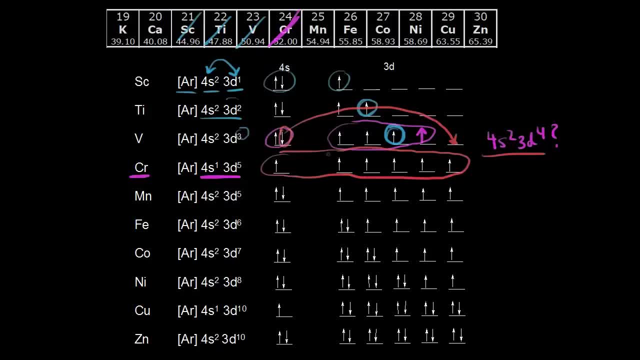 Just to make things easier when you're writing electron configurations, you can think about moving an electron from the 4s orbital over to the last empty d orbital here. Some people say that this half-filled d subshell. let me go ahead and circle it here. 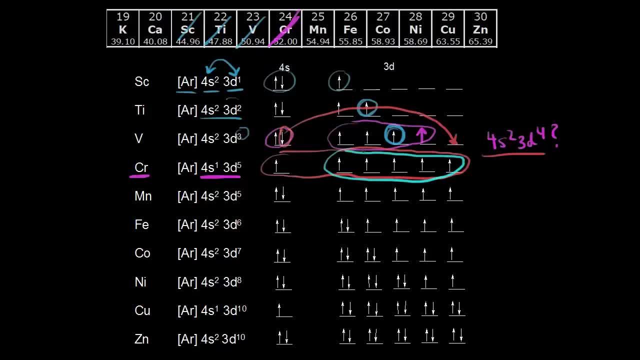 this half-filled d subshell is extra stable. That might be true for the chromium atom, but it's not always true. It's not really the best explanation. The real explanation is extremely complicated and actually just way too much to get into for a general chemistry course. 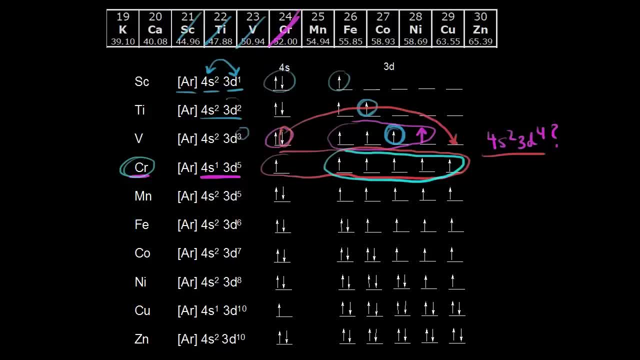 Next element is manganese. Let me go ahead and stick with blue here, Manganese. one more electron than chromium here: Chromium, we had six electrons, here, Manganese, we need to worry about seven electrons. This is kind of what we expect. 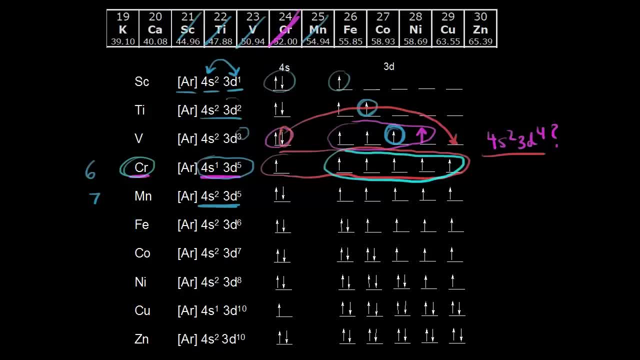 Just going across the periodic table. let me go ahead and do this for manganese. Let me use green here. You might say, okay, that's 4s1,, that's 4s2, and then 3d1,, 3d2,, 3d3,, 3d4,, 3d5. 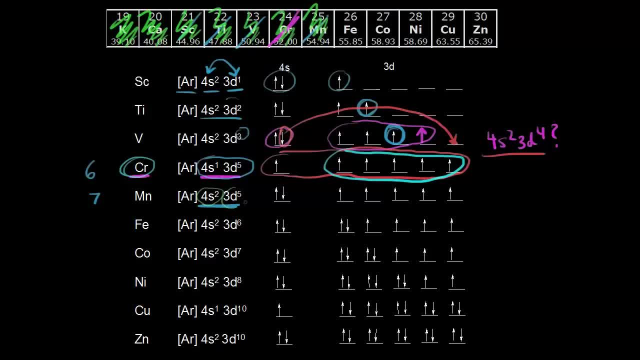 You might say to yourself: 4s2, 3d5.. This kind of proceeds how we would expect it to. The same thing with iron: 4s2, 3d6.. That takes care of iron Once again. now you can start to pair up your spins. 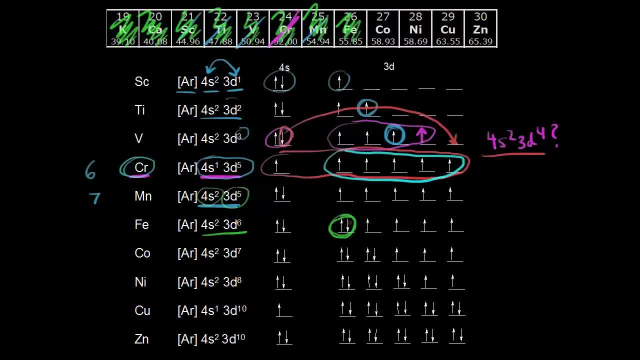 We've seen that in earlier electron configurations. Next cobalt. one more electron to worry about, 4s2, 3d7- makes sense. You can see, here would be the electron that we added and we paired up our spins again. 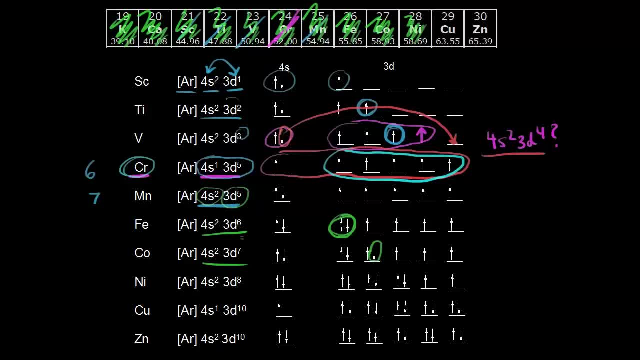 Nickel: same trend. We add one more, electron 3d8.. That makes sense. Here's the electron that we added. Once again, we get a weird one When we get to copper. copper, you might think. let me use red for copper. 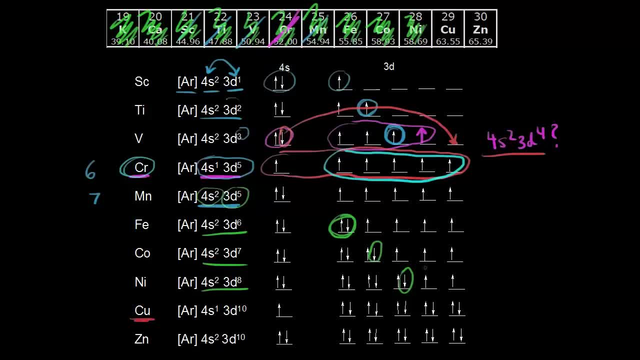 so we know copper is red. If we think about it, we're adding one more electron. If we took the electron configuration here for nickel, we added one more electron. you might guess that would be the orbital notation for copper. That's not what we see. 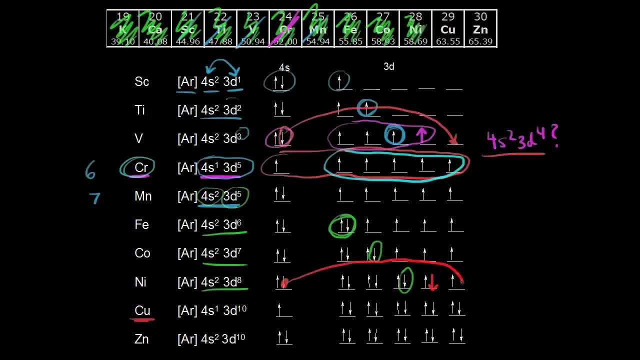 We've taken this electron here and moved it over to here like that. This gives us a filled D subshell here Once again. one explanation you'll see for that is that this is extremely stable for copper. That might be true for copper. 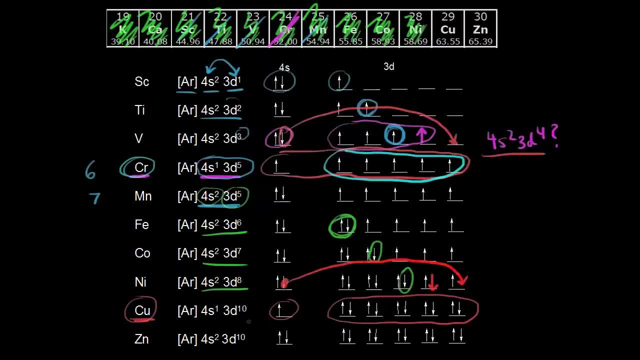 That leaves us only one electron here in our 4s orbital. The electron configuration is 4s1, 3d10.. All of these general chemistry explanations are just a little bit too simple for reality If you're just starting out. 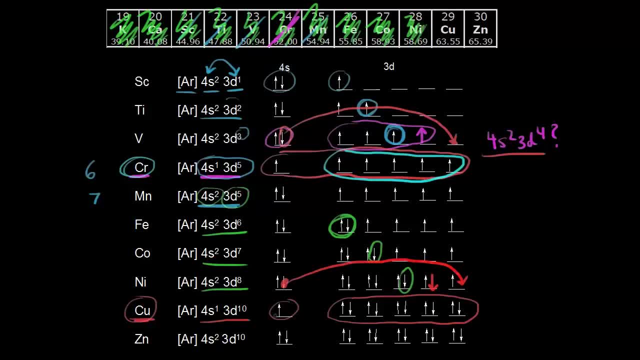 they're a pretty good way to think about it. Then, finally, zinc. Zinc makes sense. We're adding one more electron. We just took care of copper For zinc, we have one more electron. You could think about this being 4s2, right here. Then we have 3d10.. 1,, 2,, 3,, 4,, 5,, 6,, 7,, 8,, 9,, 10.. 4s2,, 3d10, or 3d10,. 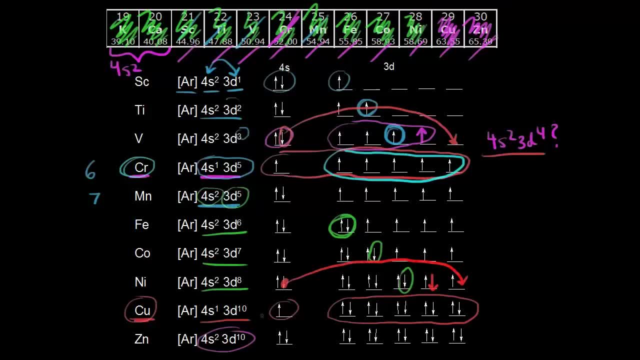 4s2 with argon in front of it gives you the complete electron configuration. You can see you've now filled your 4s orbital and your 3d orbitals- like that- Once again pretty complicated topic. Hopefully this just gives you an idea. about what's going on. 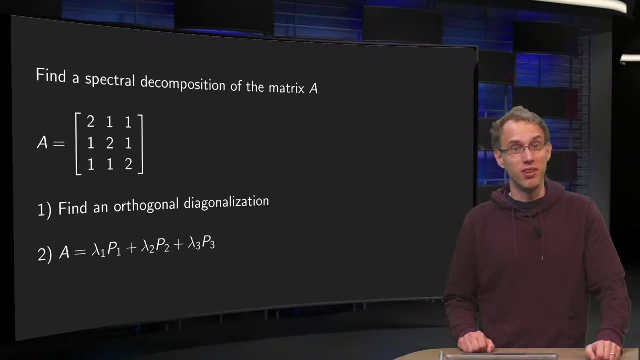 We know how to make the spectral decomposition of a matrix in theory. Let us try to do so in this explicit example. So we have our matrix A. How do we find our spectral decomposition? First of all, we need an orthogonal diagonalization, So we need the eigenvalues and eigenvectors and we have to form orthogonal bases.